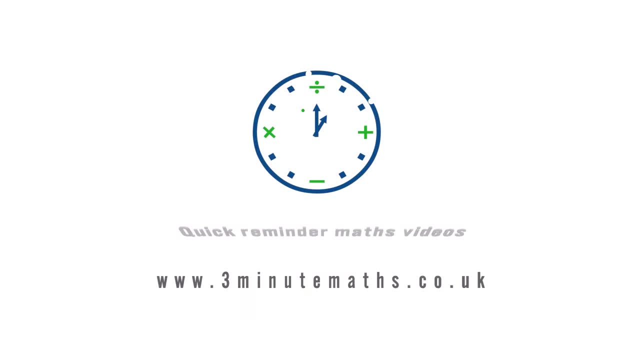 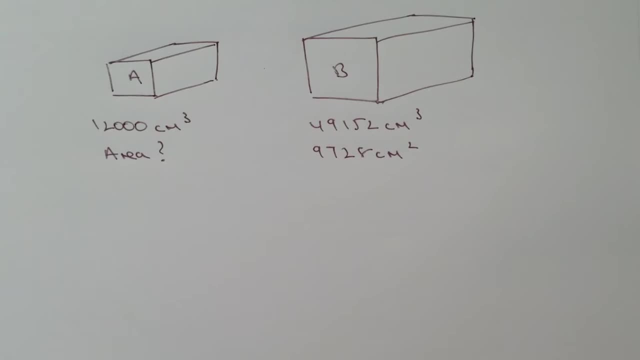 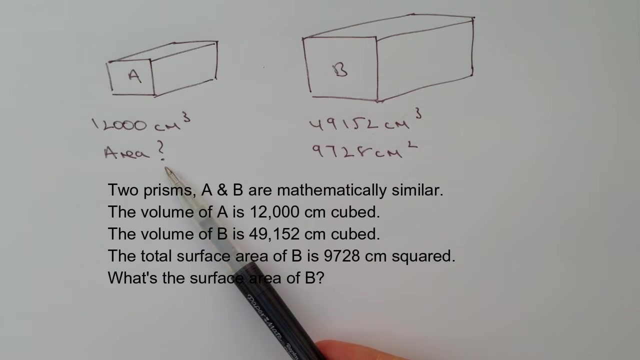 Hi, in this particular video we're asked to work out the surface area of one of the mathematical shapes which is similar to the other mathematical shapes. So the information we're given is that shape A has a volume of 12,000 cm3, shape B- 49,152, has a surface area of that. 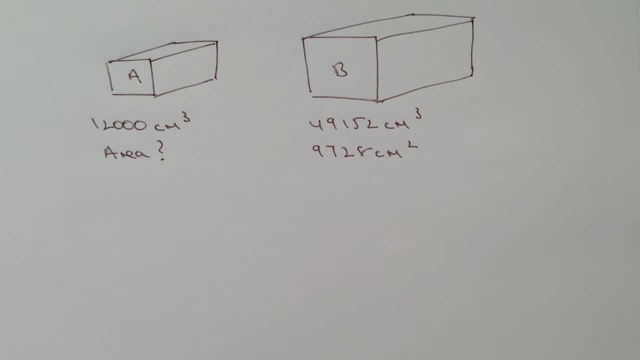 and we're asked to work out the surface area of shape A. Okay, so the numbers themselves look a little bit daunting, but really it's just a calculator question, because we're trying to establish the relationship between 12,000 cm3 and that's going to equal. 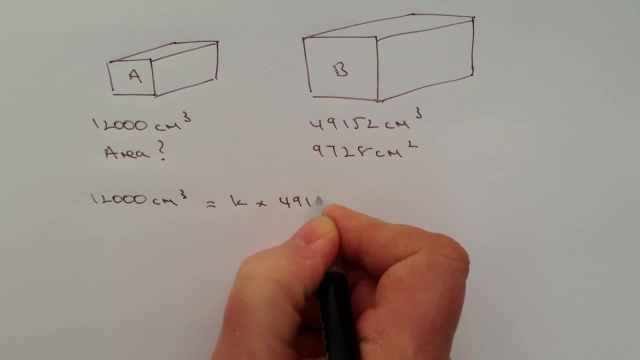 k times 49,152 cm3.. Now it is a volume relationship. so we've got to remember it's k3 and it's this constant, this scale factor, that we need to work out with these types of questions. Once we've got the value of k, then we can use it then to work out the surface area. 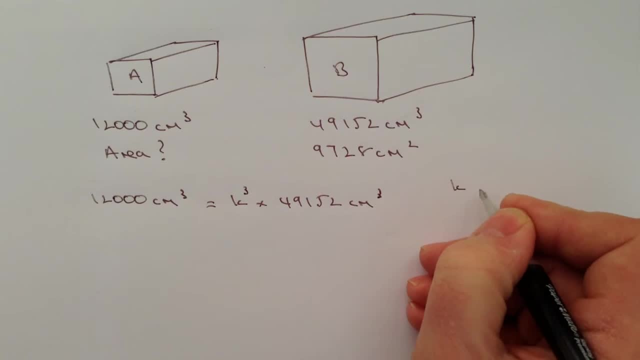 But what we have to remember is that k can either be k for linear, a linear relationship, k squared for an area or k cubed for a volume. Now, in this particular case, because we're looking at the relationship between the volumes, then we're going to use k cubed, But that's. 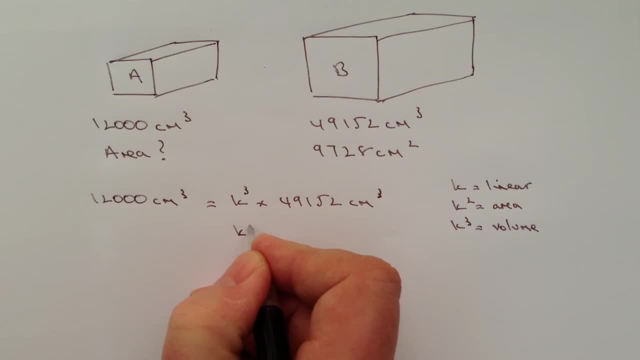 okay, because using a calculator, then we can work out the value of k cubed as being 12,000 divided by 49,152.. And then if you take that, put it into a calculator, you can see that the value of k is k squared over 49,152.. So what we're going to do is we're going to 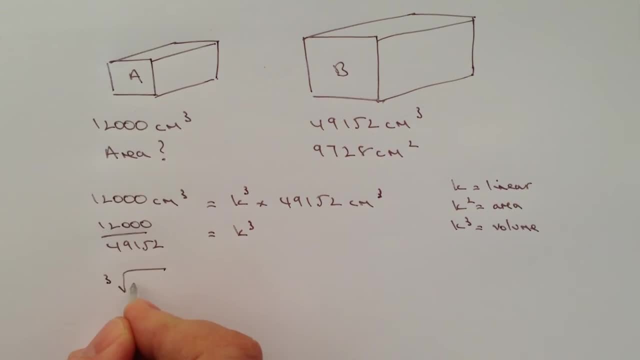 use the calculator and work out the cube root So effectively. we're looking at 12,000 over 49,152 and we want the cube root of that and that will give us the value of k. What you'll find is that that will work out quite neatly to k being 0.625.. So we've found now the linear.